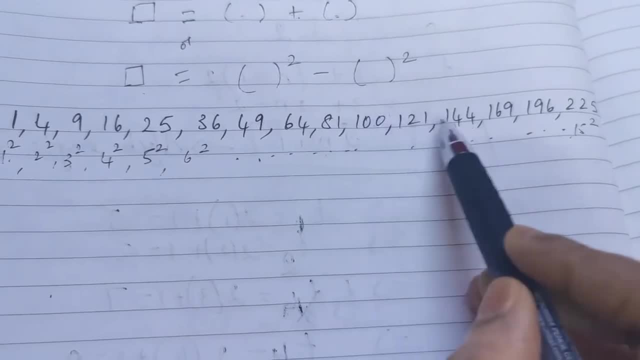 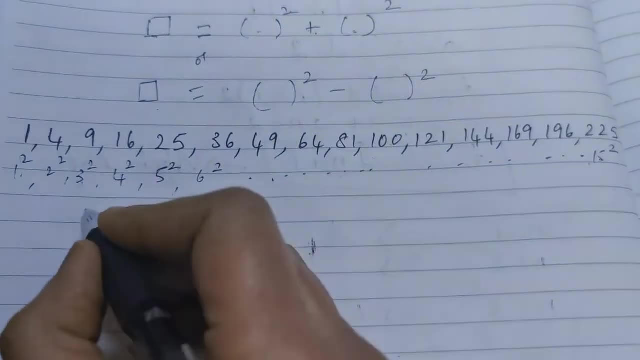 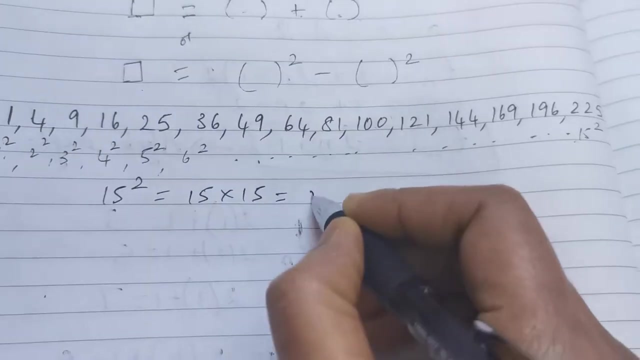 This is the square of 10,. this is the square of 11,, 12 square, 13 square, 14 square, 15 squares. Hope you know what is meant by square. 15 square means when you multiply 15 twice, you will get 25.. 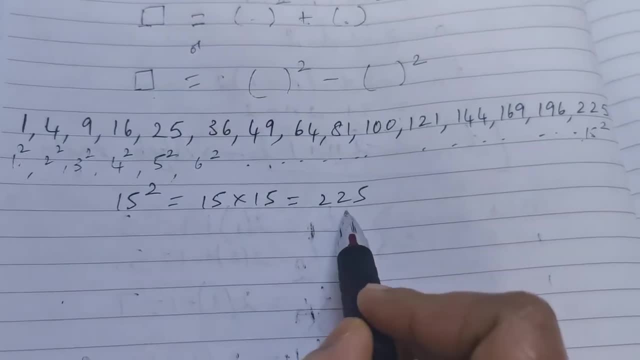 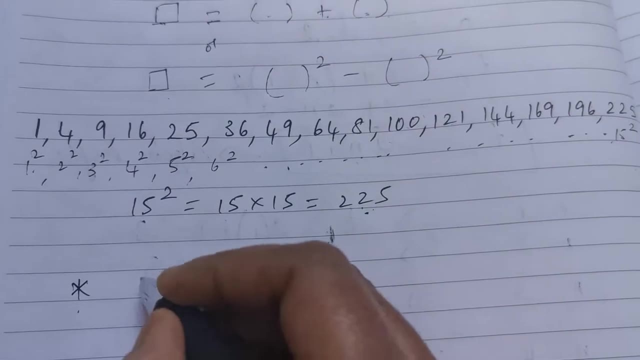 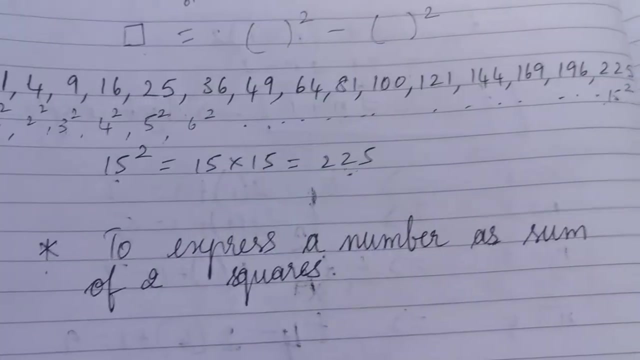 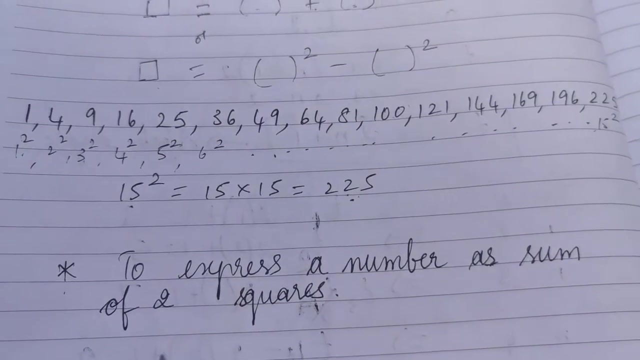 This is the meaning of square. So 225, 225 is the square of 15.. Now to express a number as sum of two squares. So first let's see how to express a number as sum of two squares. For example, I have a number 52.. 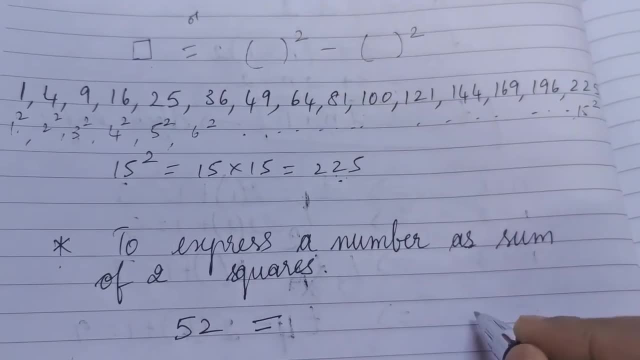 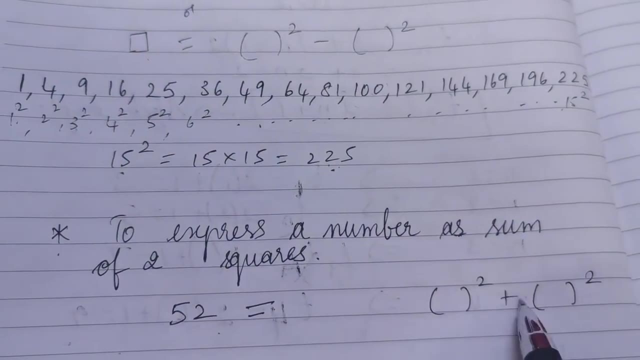 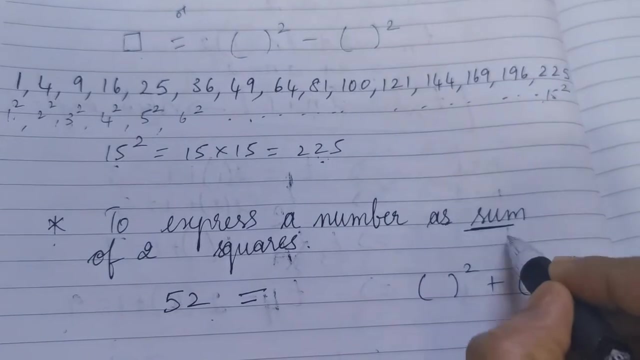 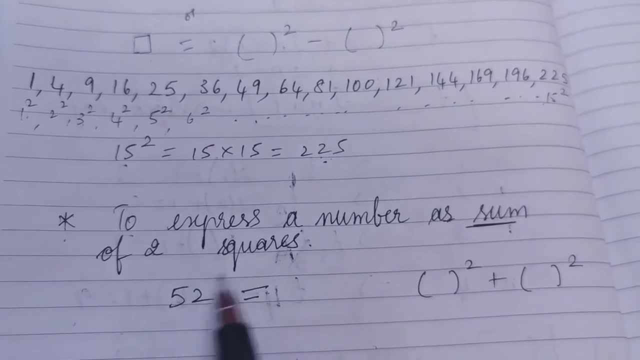 52.. This should be expressed as sum of two squares. So it should be expressed as sum of two squares. So to do this, to express as a sum, we will look for a number, look for the number which is lesser than 52.. 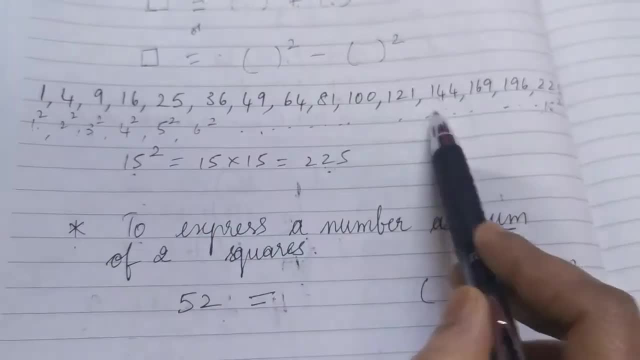 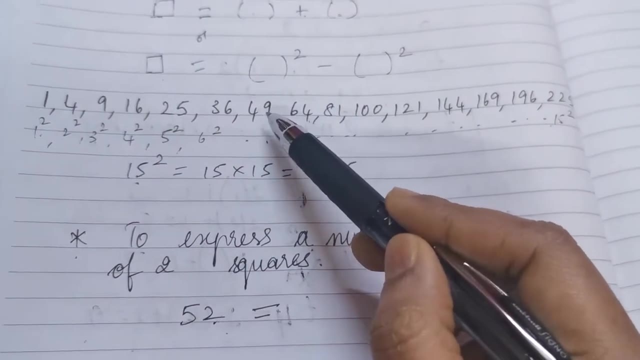 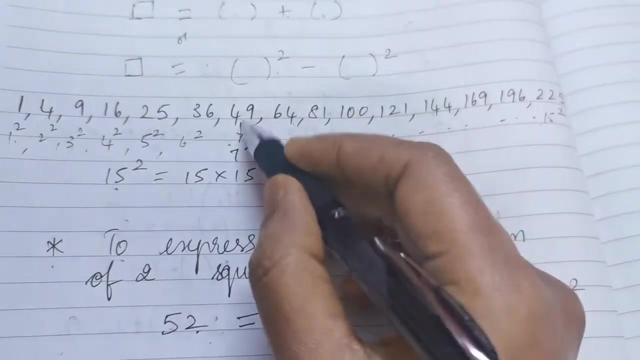 And that number should be a square number. We will look into this list- A number which is lesser than 52.. So a number which is lesser than 52 is 49.. So 49 is a square of 7.. 49 is a square of 7.. 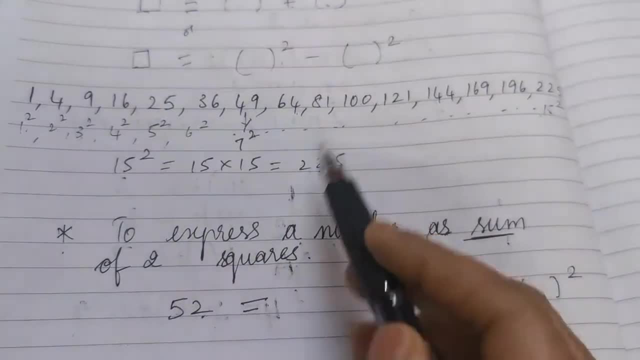 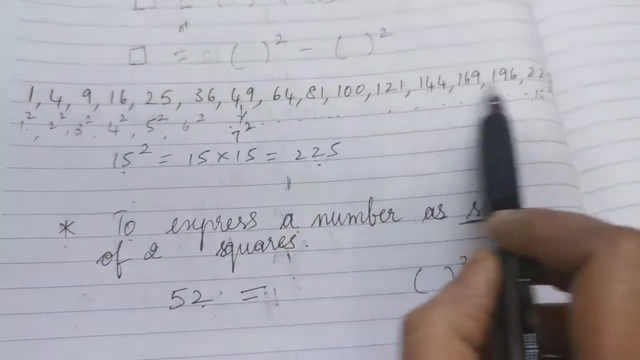 So 49 plus what will give us 52?? 49 plus 3 will give us 52.. But you cannot find 3 in this square number list. 3 is not a square number, So we cannot use 49.. 49 plus 3.. 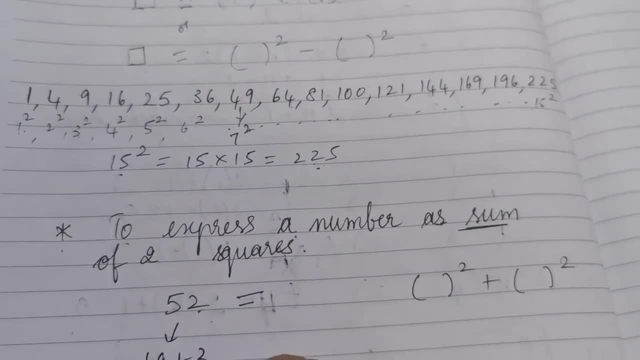 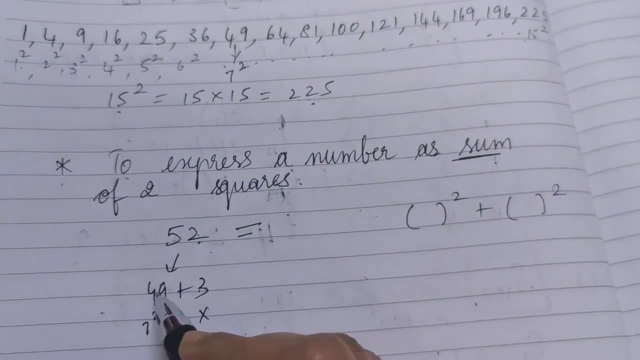 So 49 plus 3.. This is 7 square, But this is not a square number. 49 plus 3 will give us 52.. But 49 is a square number. 3 is not a square number, So we cannot apply this here. 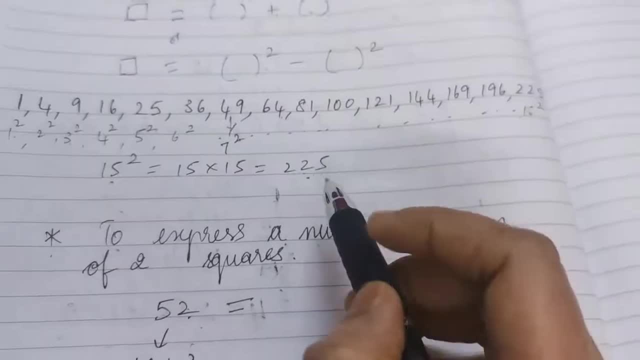 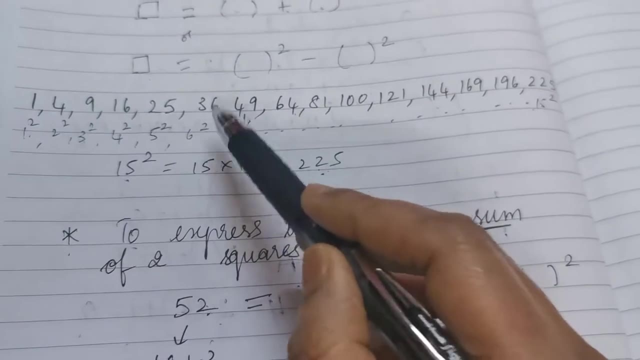 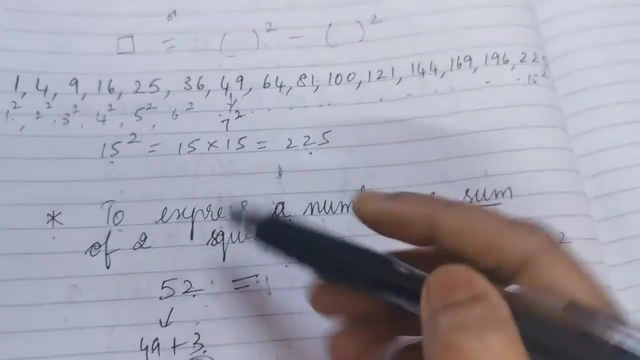 7 square plus some other square should be written. So now 49 does not work for 52.. So look into the next smaller number. So the next smaller number is 36.. So 36 plus what will give us 52?? So 36 plus 16 will give us 52.. 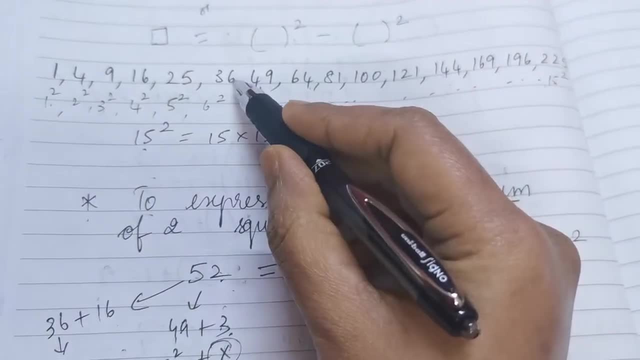 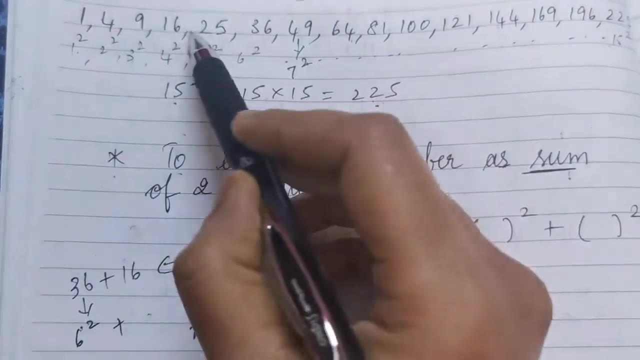 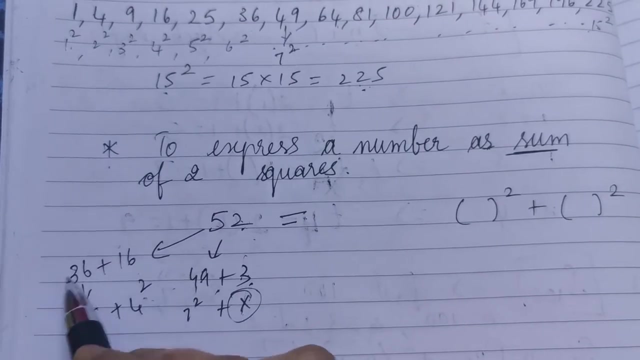 Now, is 36 a square number? Yes, It is a square of 6.. 36 is a square of 6.. And is 16 a square number? Yes, 16 is a square of 4.. So now I got both my numbers as square numbers. 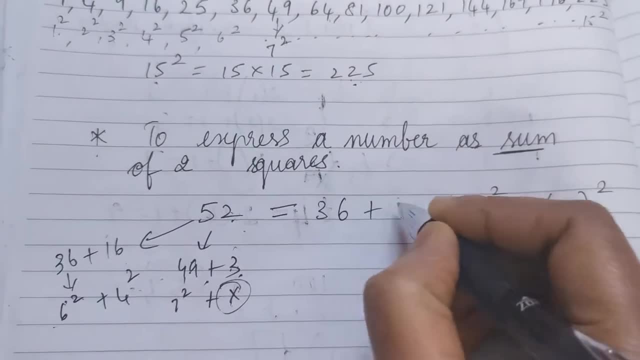 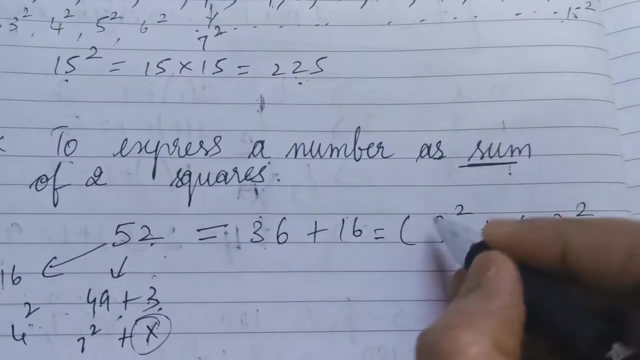 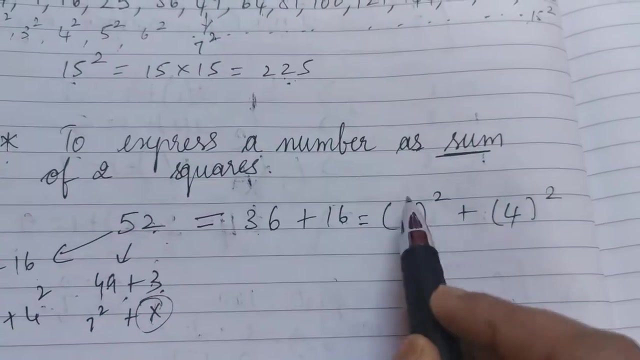 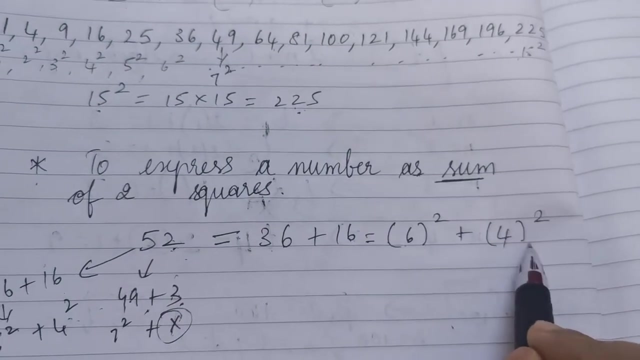 Now 52 can be written as 36 plus 16. So 36 is a square of 6. And 16 is a square of 4. So we express 52 as sum of 2 squares. So now we have 6 square and 4 square. 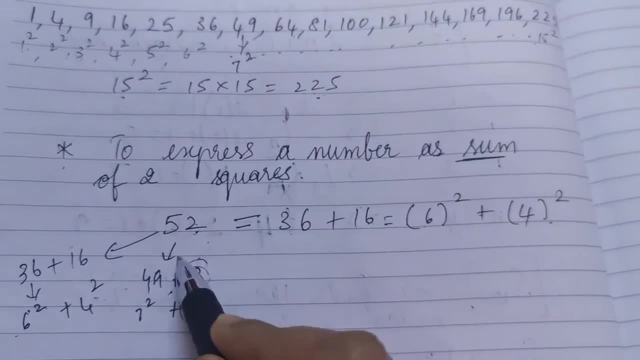 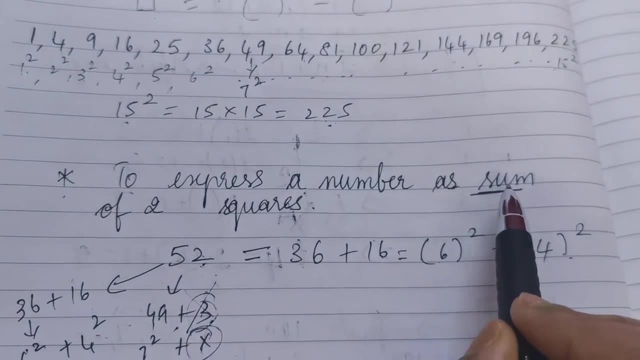 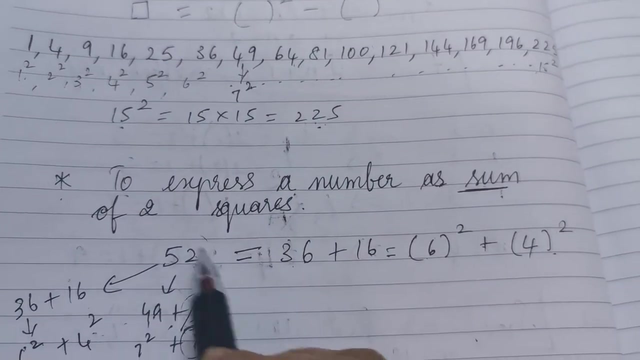 We did not take 49 and 3 because 3 was not a square number. We should take both the numbers as square numbers. So whenever we want to express a number as sum of 2 squares, look for a number which is: look for a square number which is lesser than 52.. 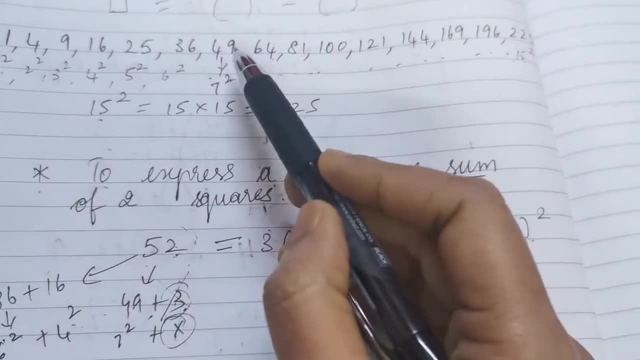 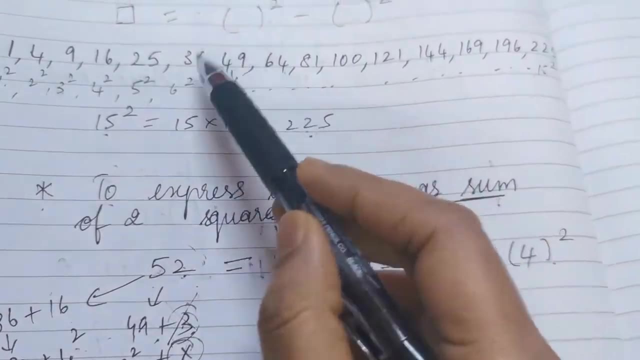 Immediately lesser than 52.. The immediate number which is less than 52 is 49.. But 49 plus 3 is 52, where 3 is not a square number. So we will look to the next number in the list, a next smaller number. 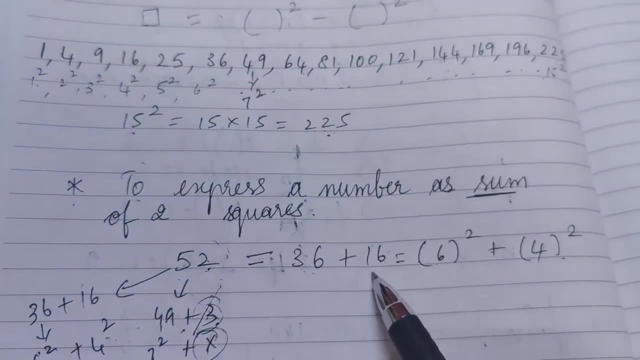 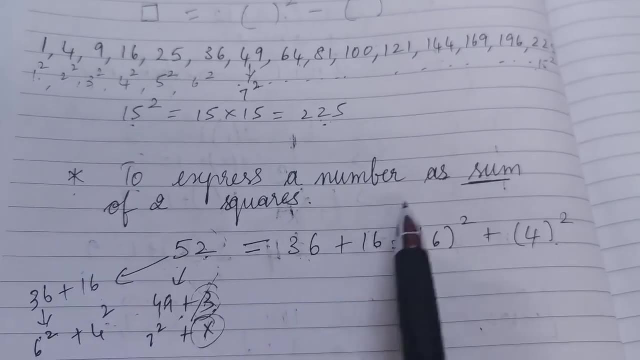 So the next smaller number, So the next number is 36,. 36 plus 16 will give us 52, where 36 and 16, both are square numbers. This is the way how we will express a number as sum of 2 squares. 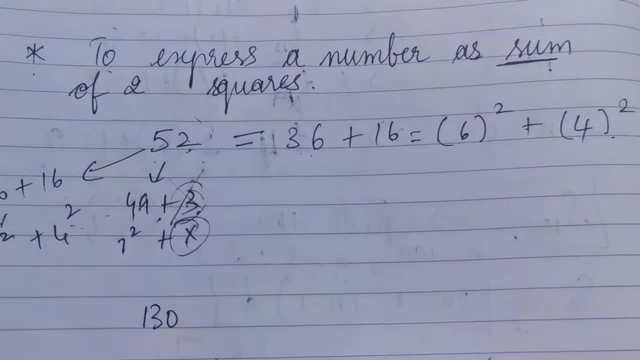 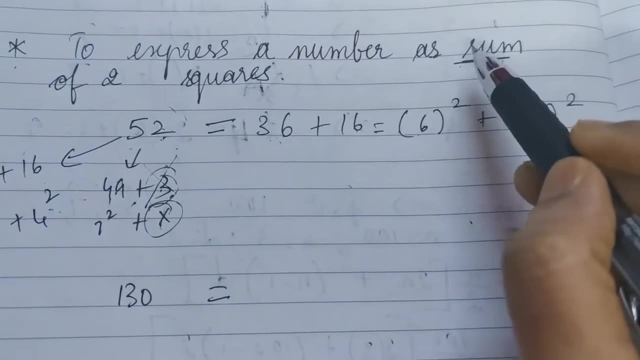 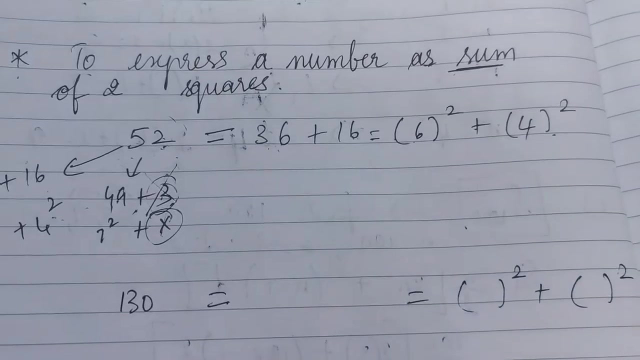 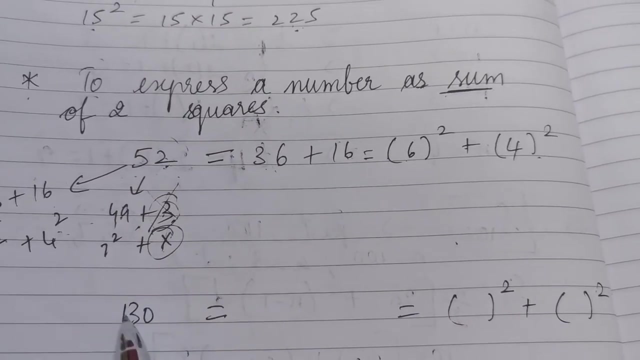 Let's try another example. So here I have another number: 130, 130, which should be expressed as sum of 2 squares. So it should be expressed as sum of 2 squares. Now the procedure for this is: we will look into the list for finding out a number. 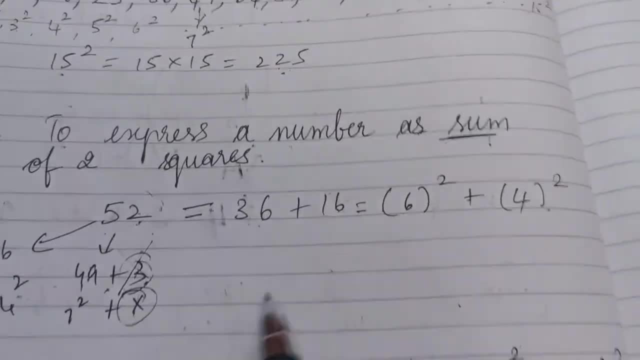 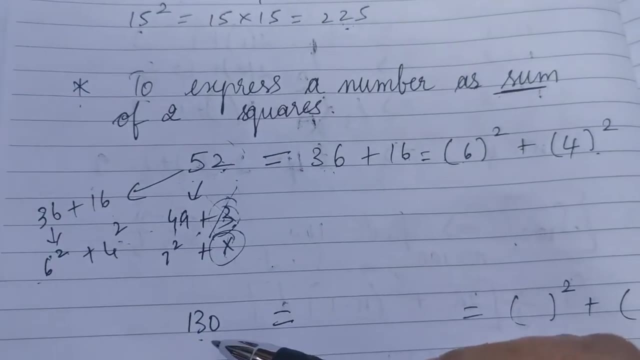 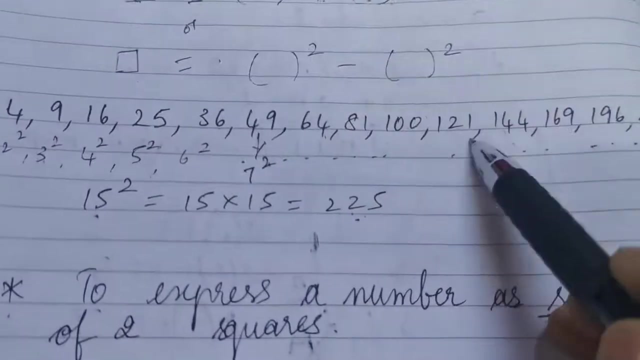 a square number which is smaller than 130.. So in this list, in the square numbers list, we will always look into the square numbers list. So look for the number which is lesser than 130.. So a number which is immediately lesser than 130.. 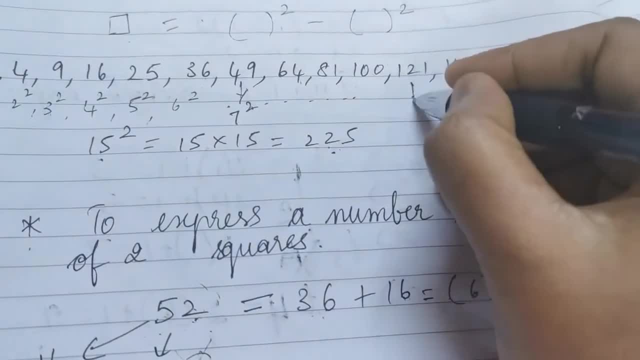 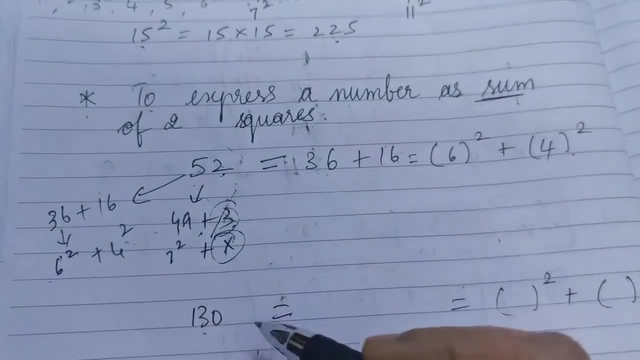 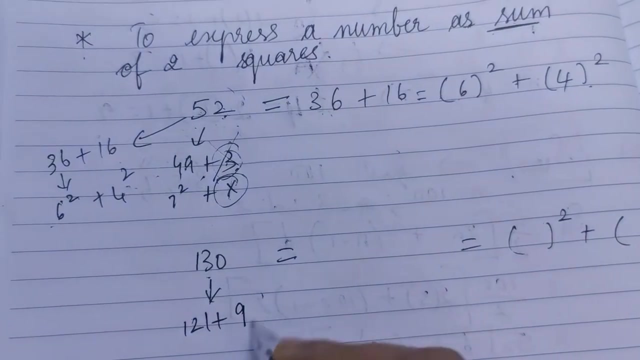 130 is 121, 121 is a square of 11.. So 121 plus what will give us 130?? So 121 plus 9 will give us 130.. So this is 11 square. what about 9?? Is it a square number? 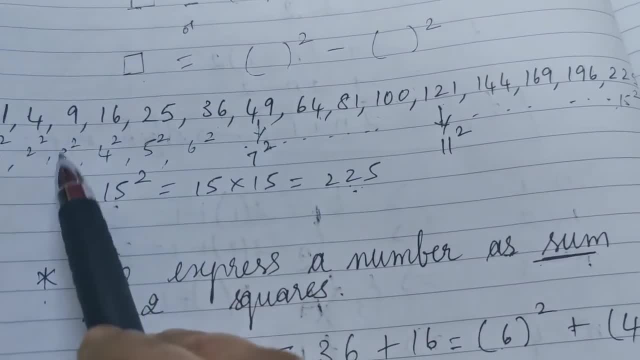 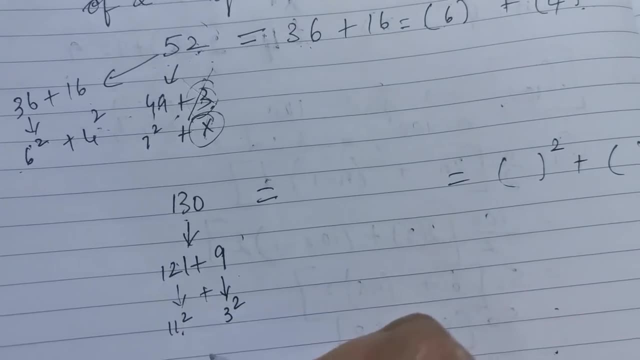 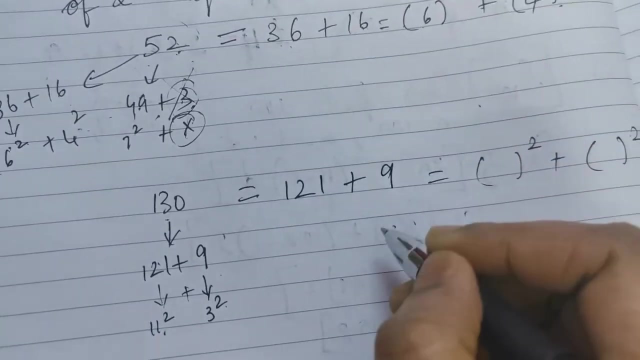 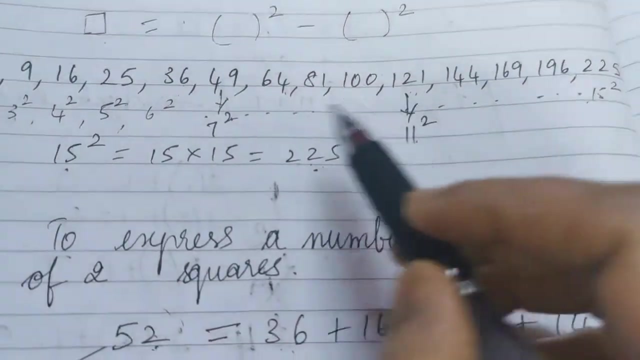 Yes, 9 is a square of 3.. So This is 3 square, So 121 and 9.. So 121 plus 9 is 130.. So 121 is the square of 11 and 9 is the square of 3.. 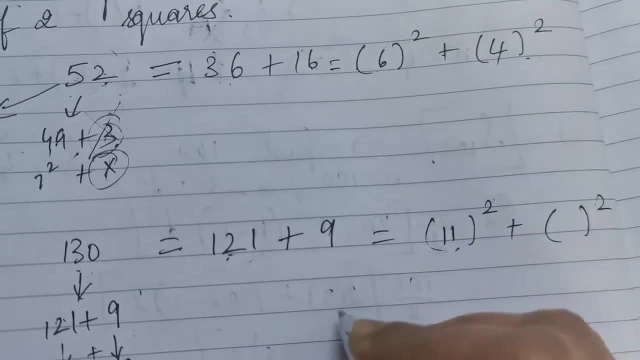 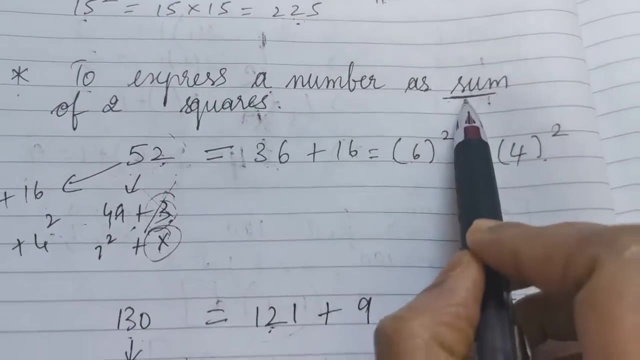 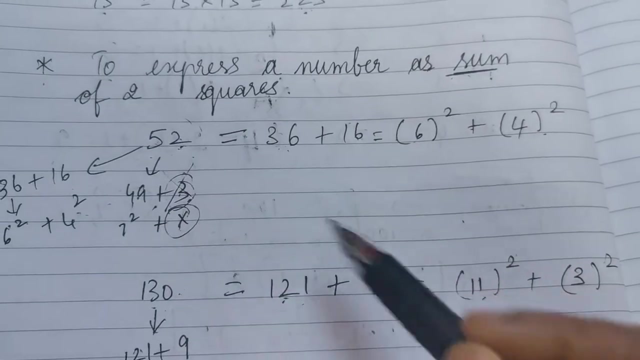 So 121 is the square of 11 and 9 is the square of 3.. So, So for expressing a number as sum of two squares, find the square number which is immediately lesser than the given number and check whether the next number you get is also a square. 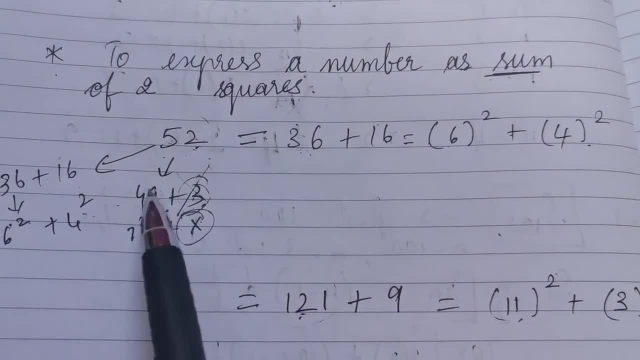 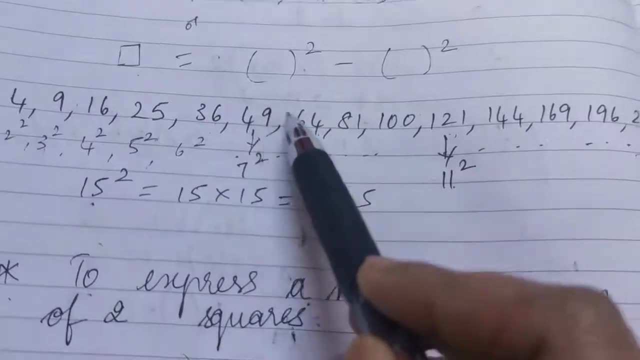 If the next number you get is not a square, as in this case. So 49 plus 3 is 52.. The second number was not a square, So look for a number smaller than that. So a number smaller than 49 is 36.. 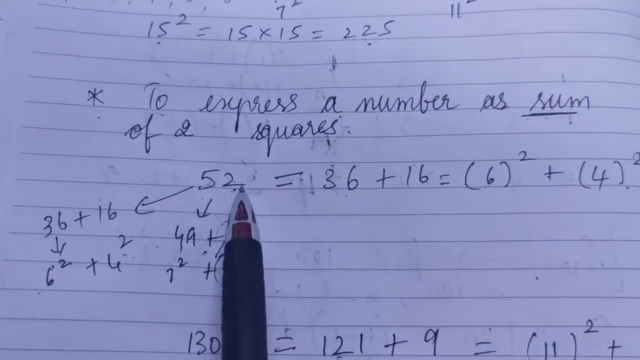 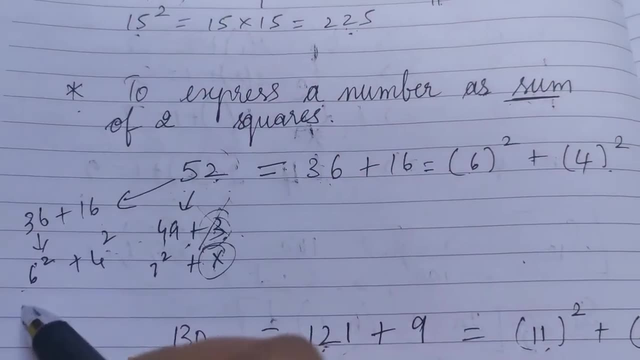 So we will look for 36.. 36 plus what will give us 52.. 36 plus 16, which is also a square number, gives us 52.. So we go for this and not for this, because 3 is not a square number. 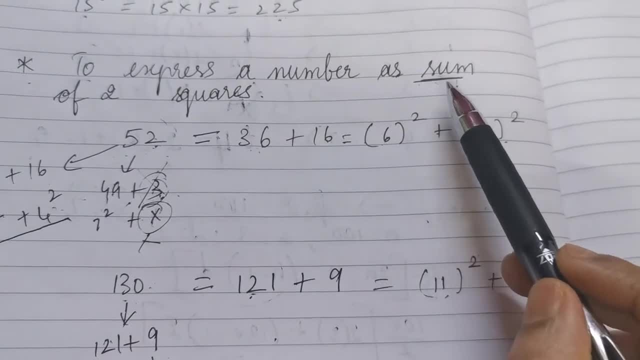 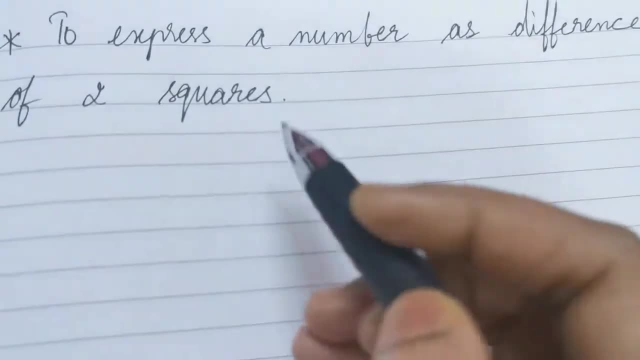 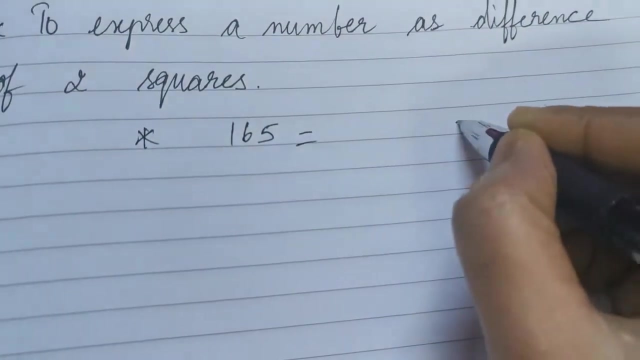 So remember this. Next, we will try to express a number as difference of two squares. So now let's try to express a number as difference of two squares. So, for example, I take the number 165.. I should express it as difference. 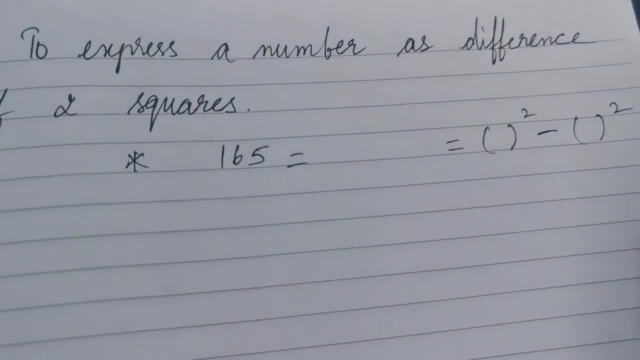 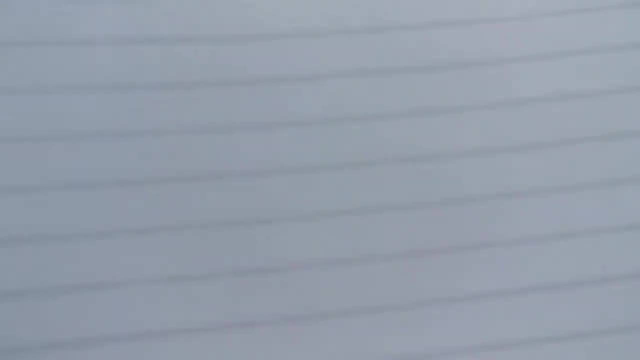 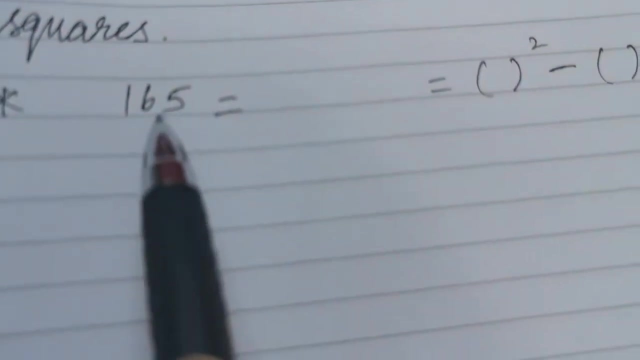 So, for example, I take the number 165 and I should express it as difference of two squares. So when it was sum, we check for a number smaller than the given number, But to find the difference we go for the opposite. We will look for a number which is greater than 165.. 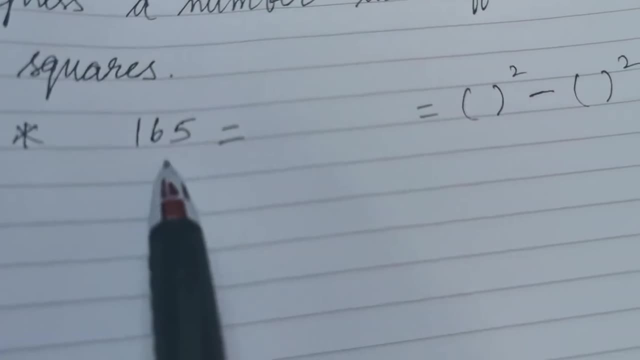 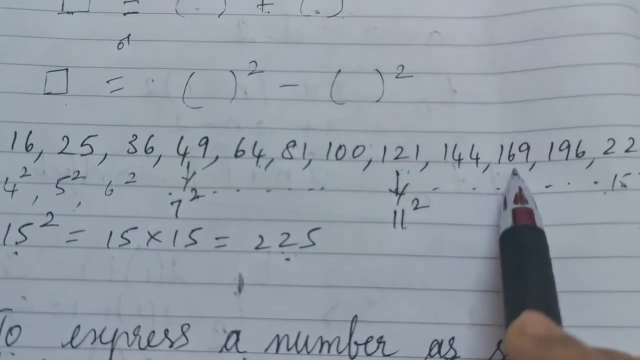 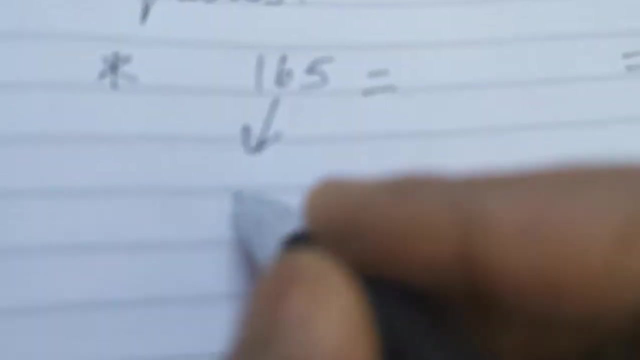 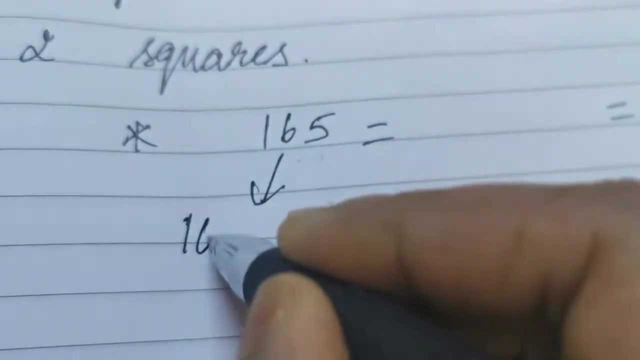 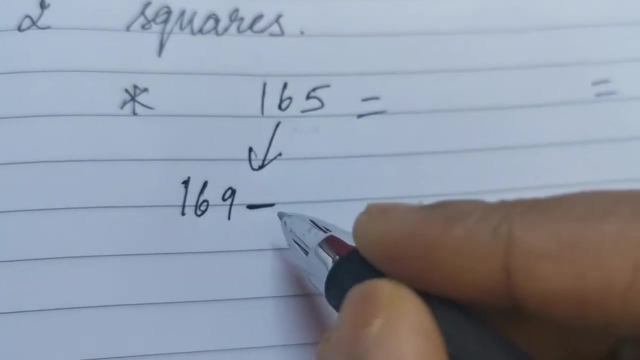 165 in the square numbers list. So a number greater than 165 here is 169.. So 169 minus what will give us 165?. So the square number we are taking here is 169.. 169 minus what will give us 165?. 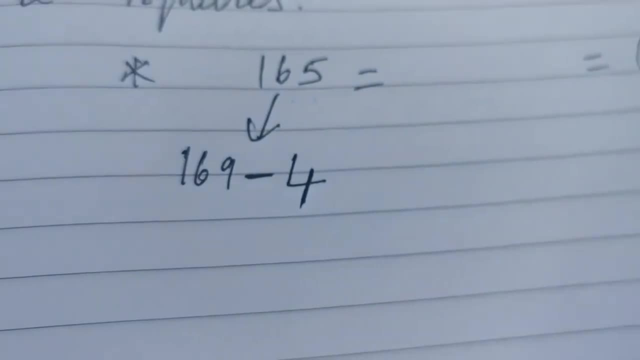 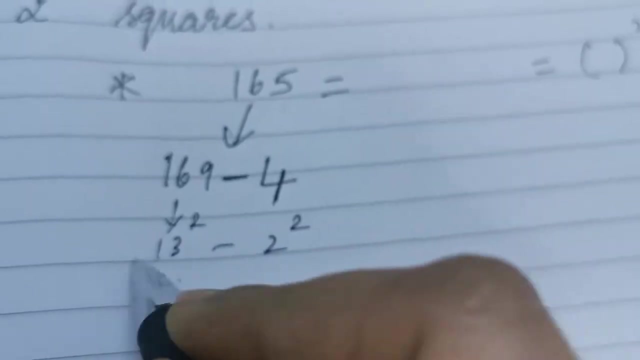 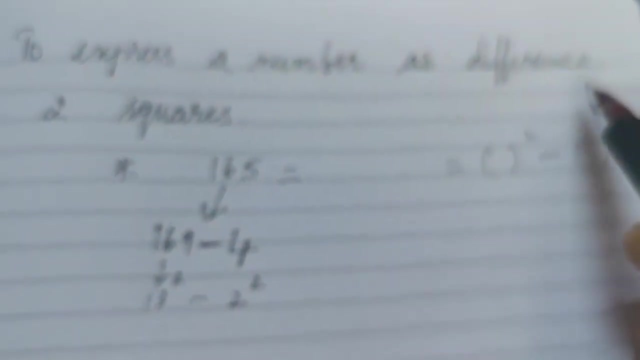 So 169 minus 4 will give us 165.. So this is a square of 13.. And this is a square of 2.. So both are square numbers. So to find, to express a number as difference of two squares, to express a number as difference of two squares. 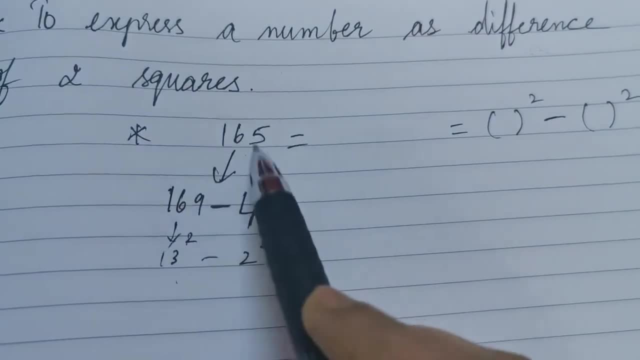 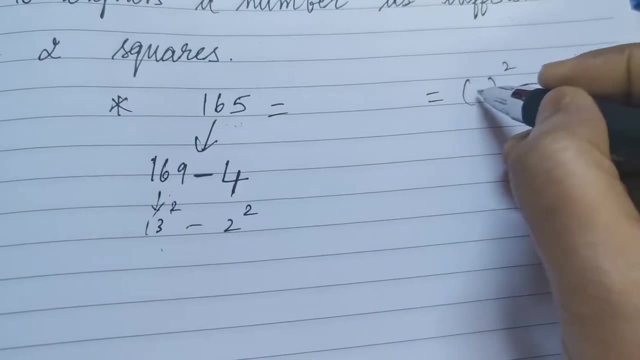 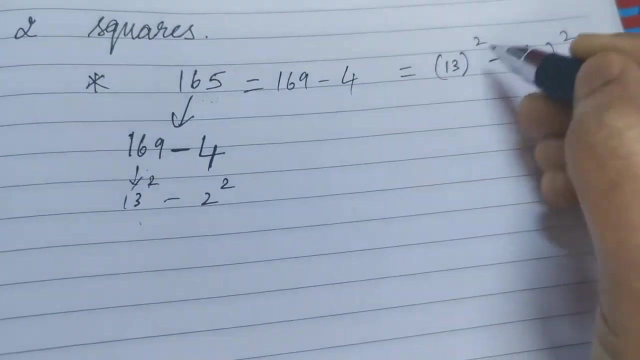 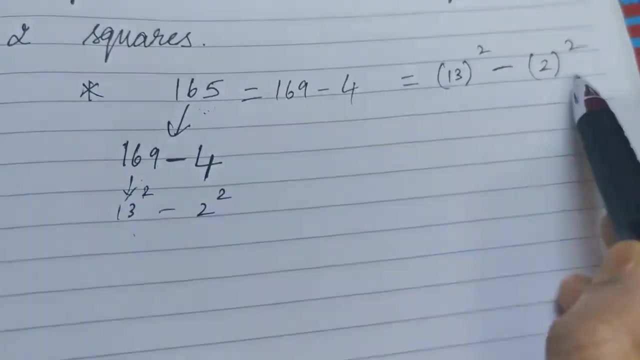 we will always look for a number greater than the given number, So I opted for 169.. So 169 is the square of 13.. 169.. 169 minus 4.. So 13 square minus 2 square. Now we expressed 165 as difference of two square numbers. 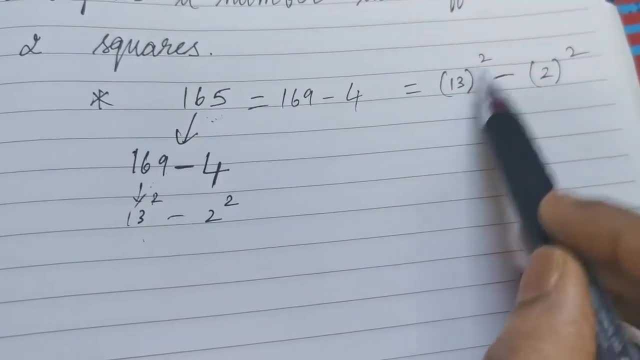 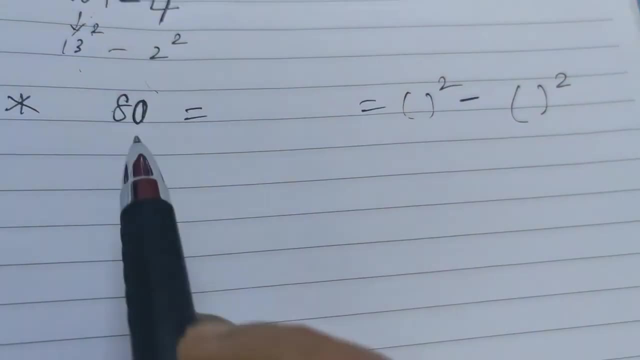 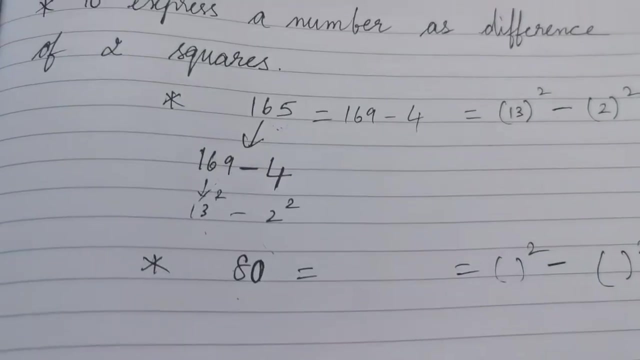 So difference of two squares, So 13 square minus 2 square. Let's try another example. So here I have a number, 80, which is to be expressed as difference of two squares. So I have to, So I have to express 80 as difference of two squares. 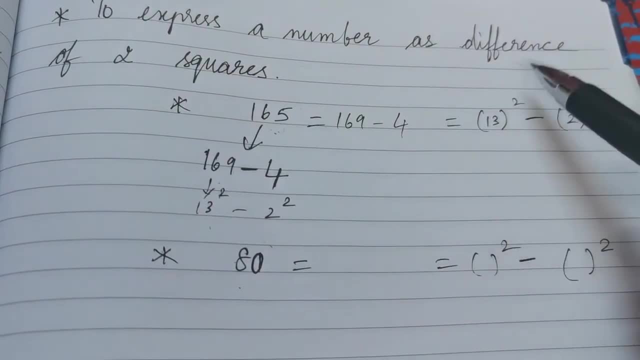 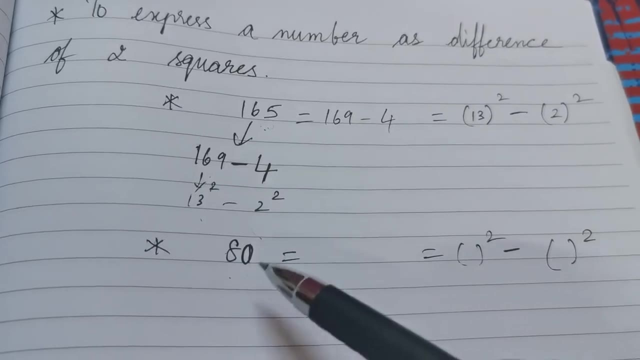 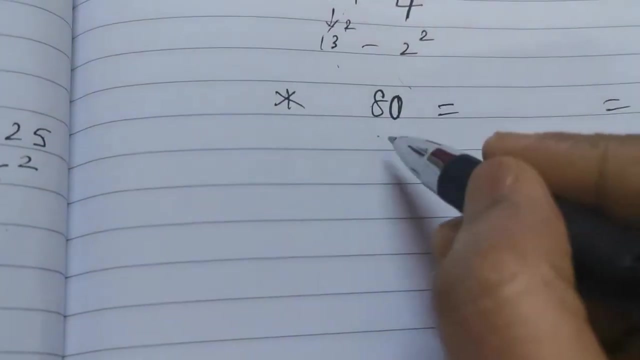 So remember to find to express a number as difference of two squares. I will look for a number which is greater than 80 in the square number list. So a number which is greater than 80 is 81.. So 81 minus. so difference means minus. 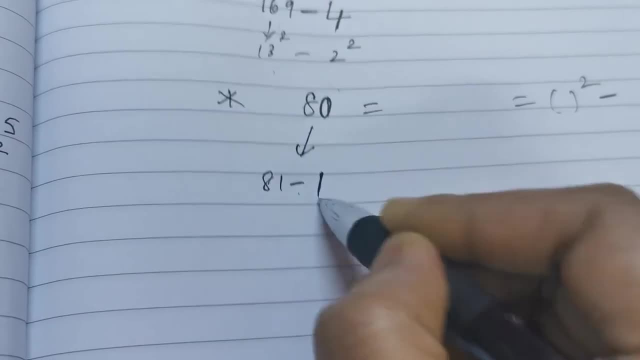 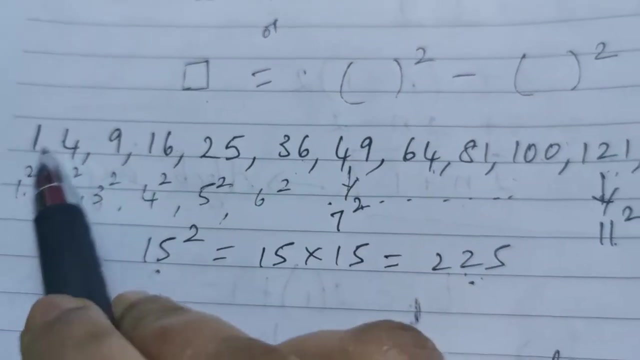 81 minus what will give me 80?? 81 minus 1.. 81 will give me 80.. Is 1 a square number? Yes, of course 1 is a square number. 1 is the square of 1 itself. 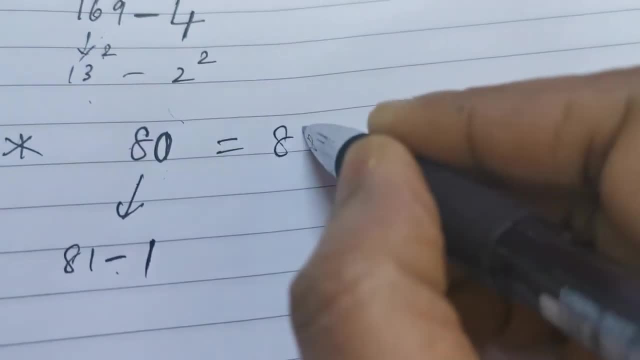 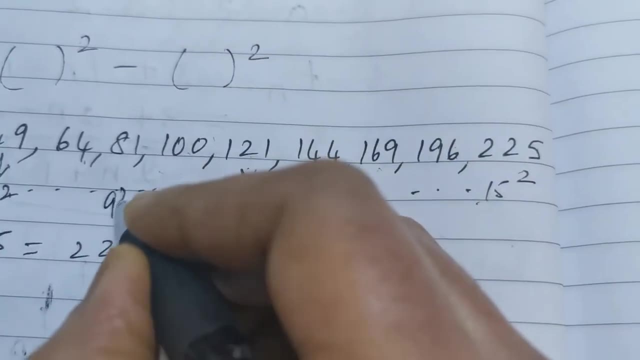 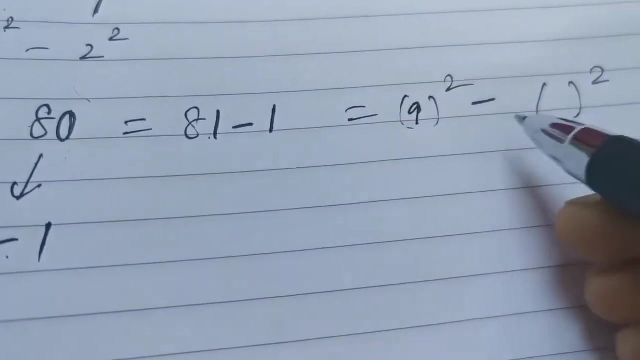 So 80 can be expressed as 81 minus 1.. 81 is the square of 9.. 9 square is 81.. And 1 is the square of 1 itself. So 9 square is 81 and 1 square is 1.. 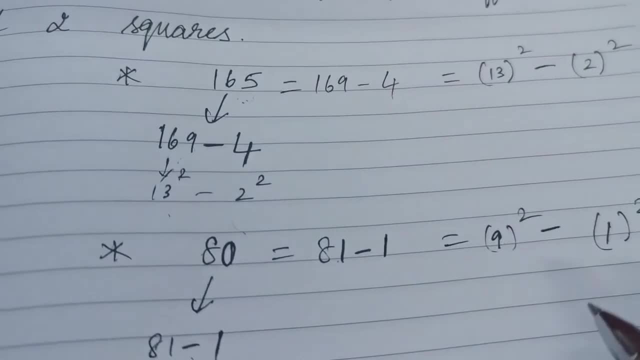 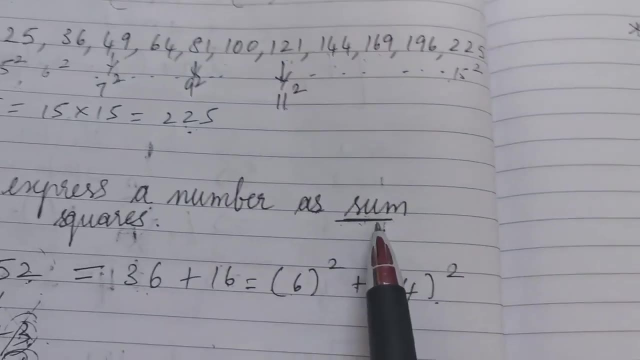 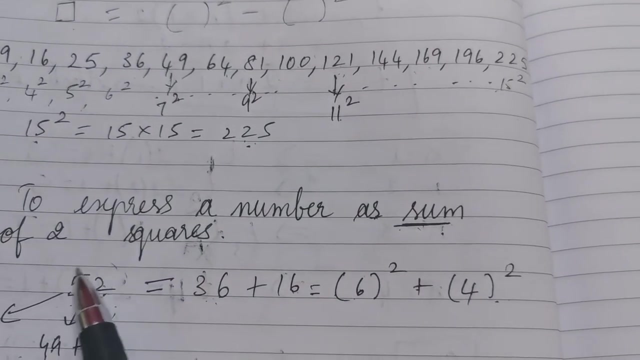 So 81 minus 1 is 80.. This is how we will express a number as difference of two squares. So let me remind you to find I am sorry to express a number of number as sum of two squares, We will look for a number smaller than the given number from the square number list. 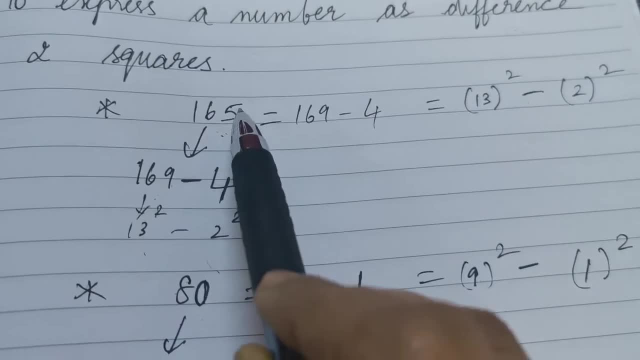 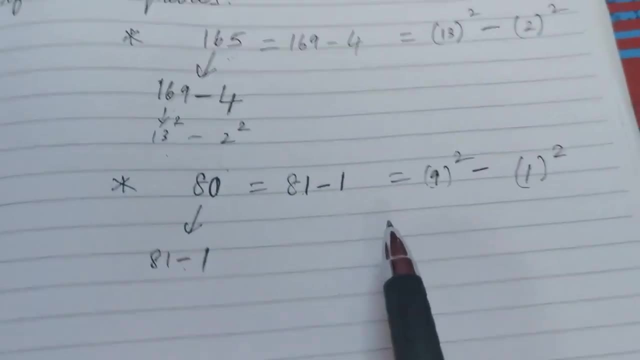 But to express a number as difference, we will look for a number which is greater than the given number from the square number list. This is the difference. So thank you. 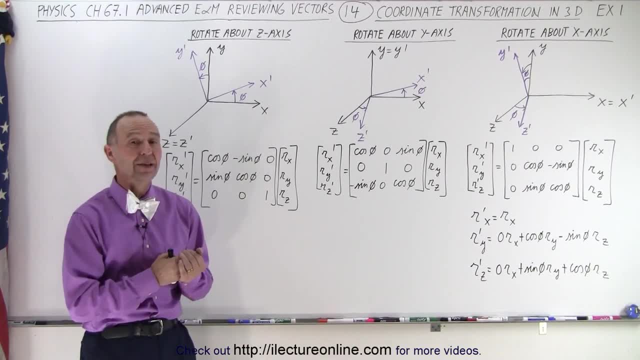 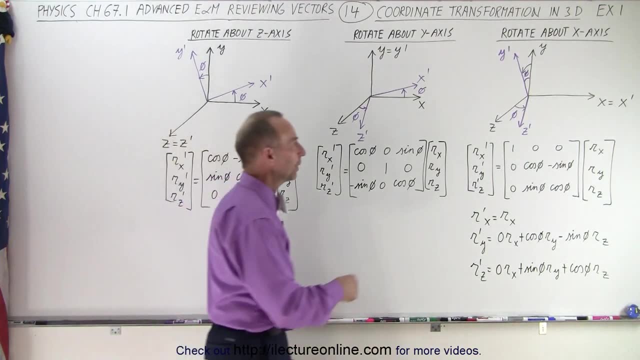 Welcome to Electron Line. Here before us we have examples of three transformations in the XYZ coordinate system. So the black lines here are the X, the Y and the Z axis. In the first case we're going to rotate about the X axis. 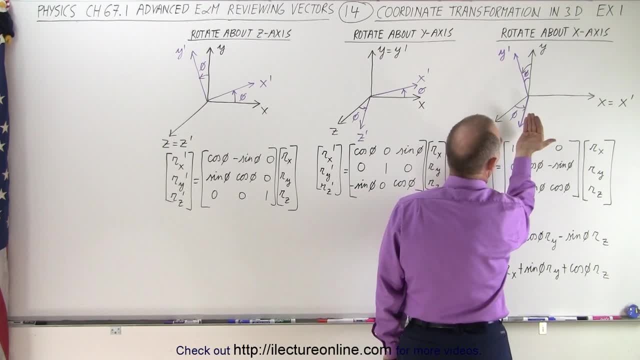 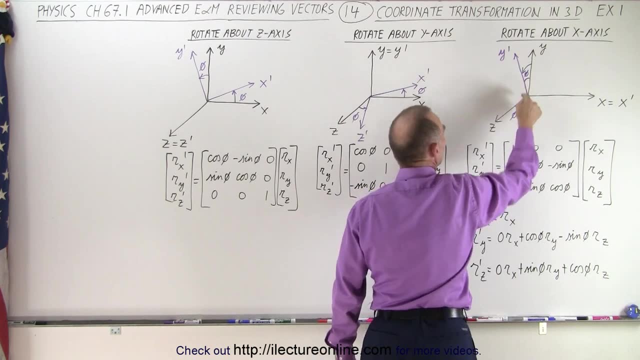 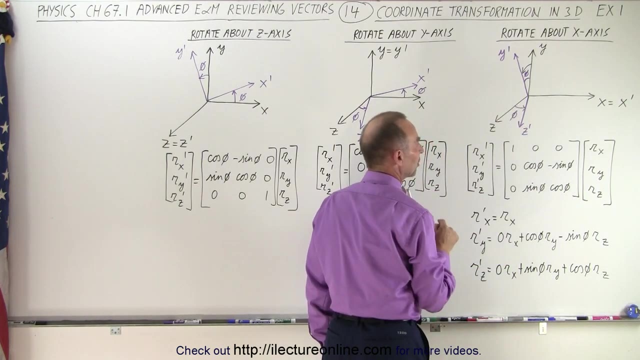 So if you put your thumb in the direction of the X axis, notice that the Y axis and the Z axis will rotate like this. So Y is going to come down and Z is going to go down as well, And we rotate it to the angle of phi, and then we have the transformation matrix right here, which represents that particular transformation. 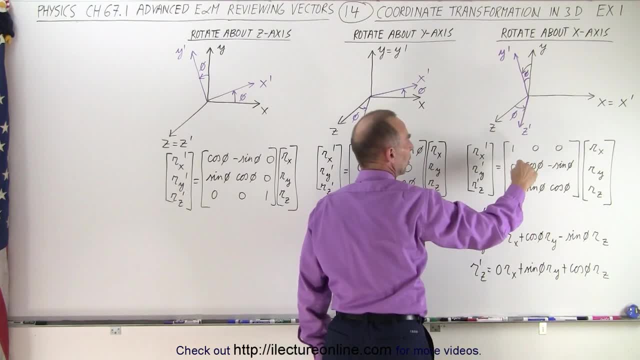 Since the X and the X prime axis are in the same direction. notice we have a 1 here and 0s here and 0s there If we now multiply the RX prime, RY prime and RZ prime with the transformation matrix, or when we take that back. 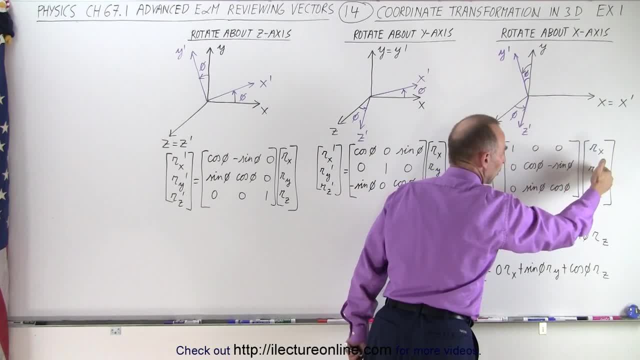 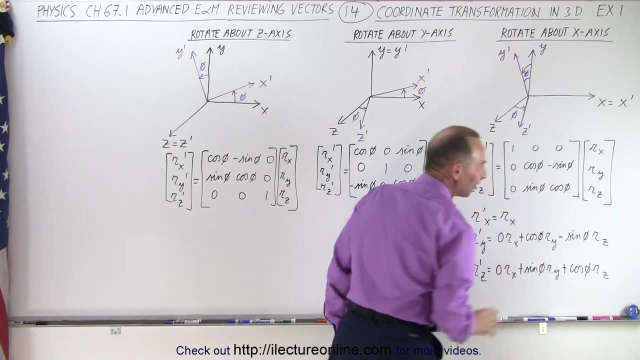 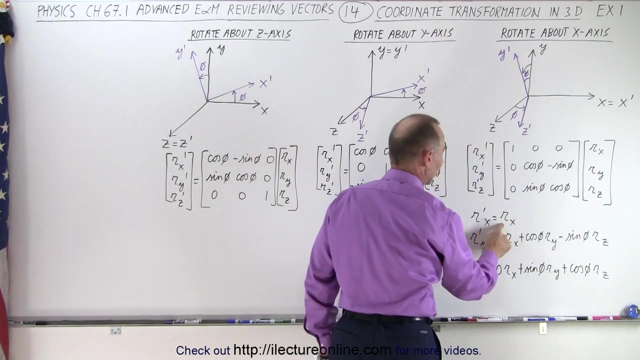 when we take the transformation matrix, we multiply it times the RX, RY, RZ matrix And we get the same vector now expressed in the transformed coordinate system. And so what we did then is we multiply this row times this column to get the first equation.